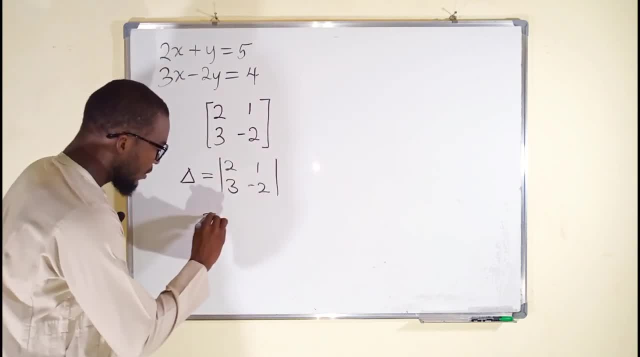 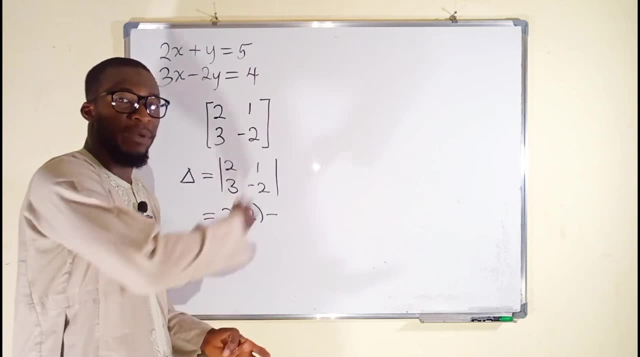 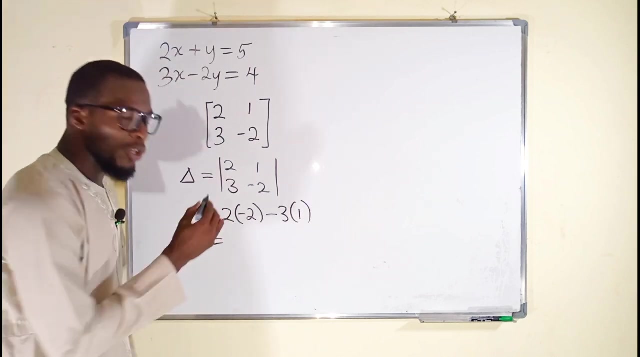 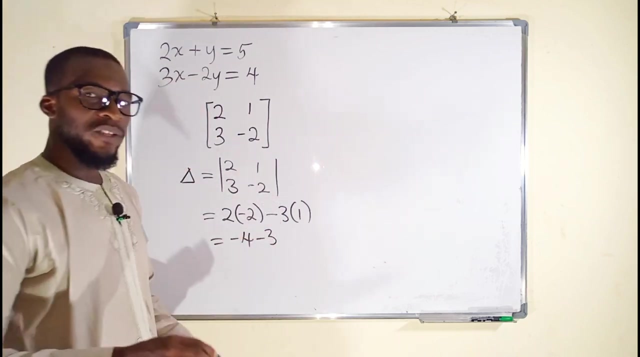 using these absolute strokes, Multiply the leading diagonals. We have 2 multiplied by negative 2.. Then you subtract. you multiply the other diagonal. We have 3 multiplied by 1.. You simplify: 2 multiplied by negative, 2 is negative 4.. Minus 3 times 1 is also 3.. 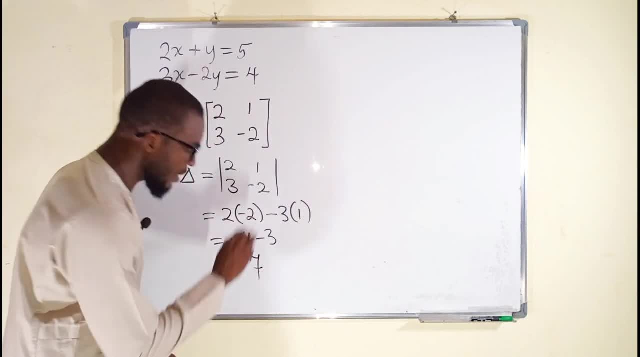 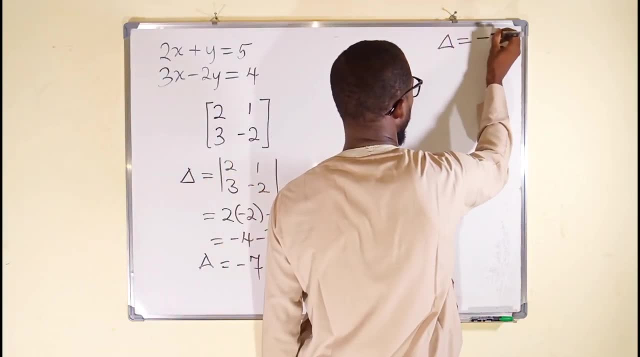 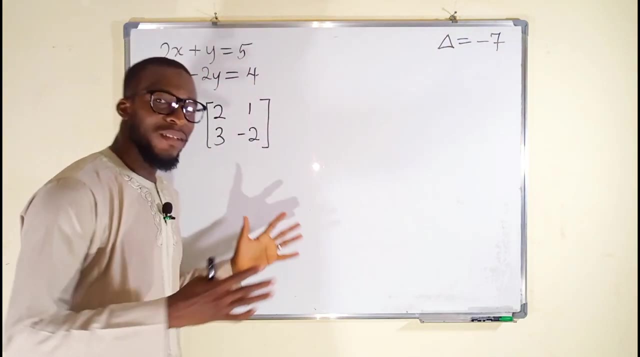 Minus 4, minus 3 is equal to minus 7.. So this is our determinant. Let us keep it aside. Determinant is equal to negative 7.. Let me wipe it away. Next, we are going to find the determinant with respect to x To. 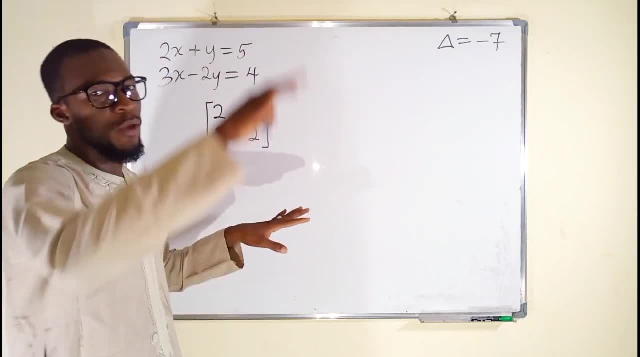 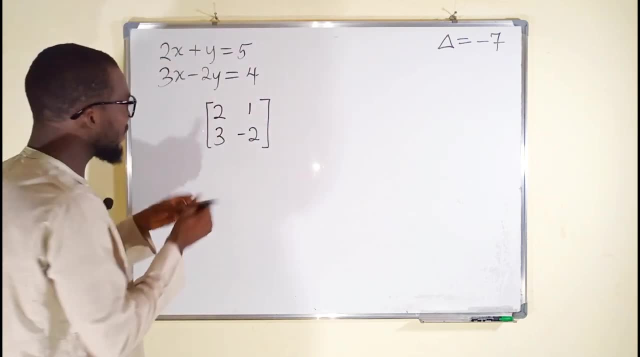 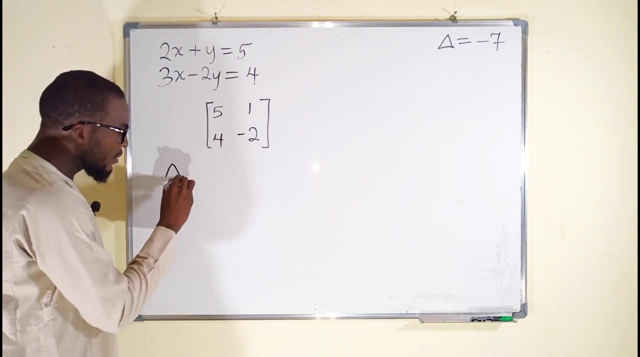 do that. we are going to replace the x column by the constant times. These are the constant 5 and 4.. These are the x column. You can see them here. We are going to replace them with constants. We have 5 and 4.. So the determinant with respect to x will be 5.. 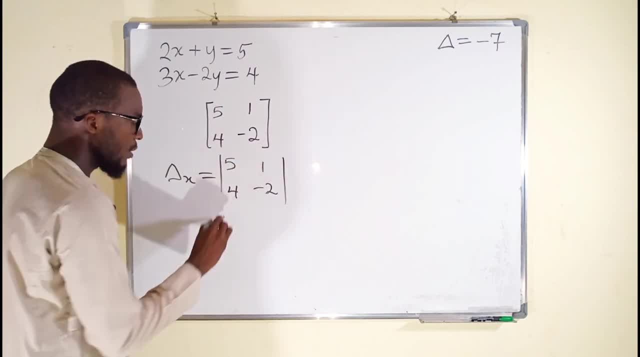 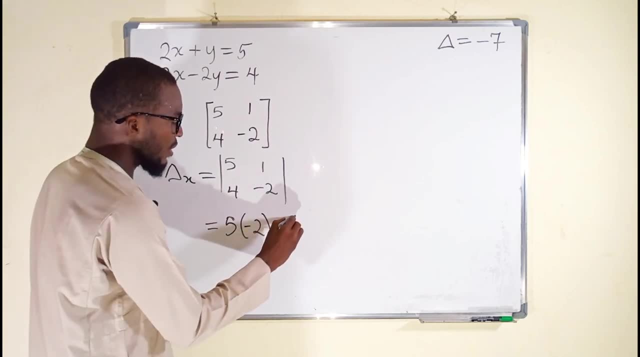 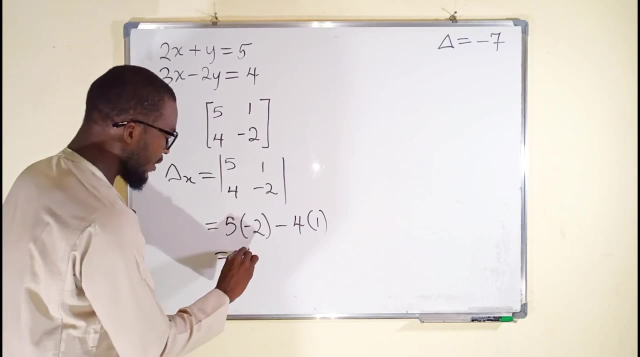 So x is equal to x to the power. 4 minus 1 is equal to negative, 2.. Let us find the determinant 5 times negative, 2.. Then you subtract 4 multiplied by 1.. Let us simplify: 5 times negative, 2 is negative, 10.. Minus 4 times 1 is 4.. Finally, the determinant: 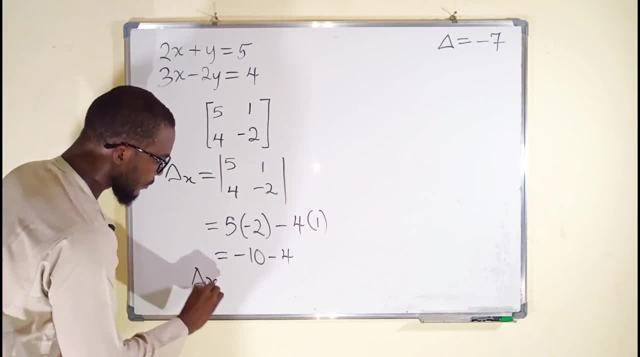 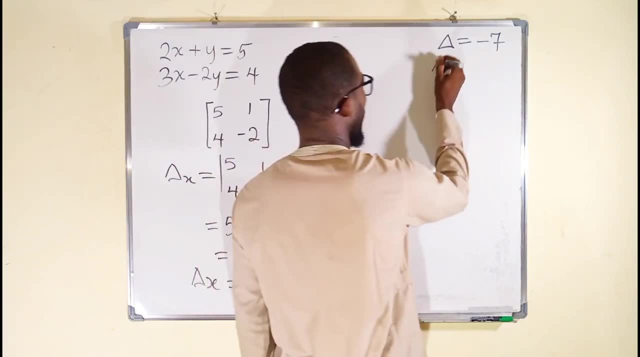 with respect to x is equal to negative 14.. You multiply that by 1.. This is our determinant. So we have 2 multiplied by x and we have 4 multiplied by 1.. This is our determinant. let us keep it aside. we have determinant with respect to x is equal to negative 14. 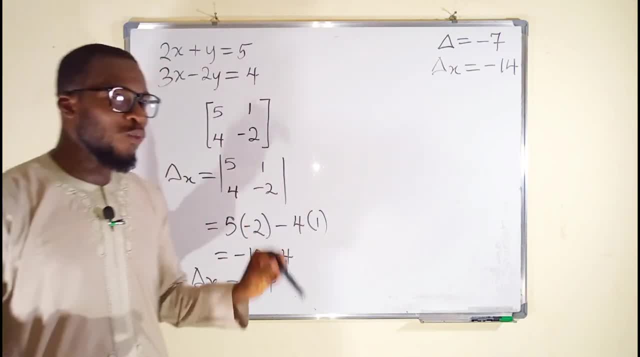 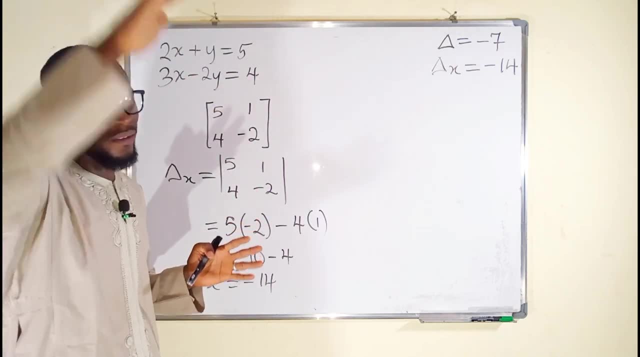 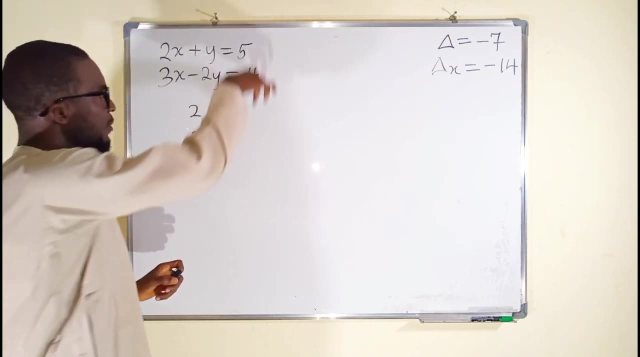 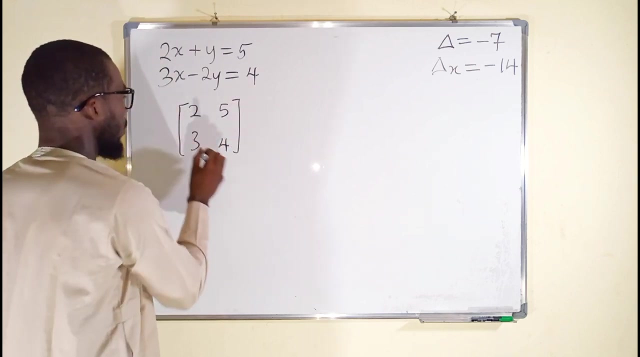 now let us find the determinant with respect to y. in this case, we are going to leave the x column constant. they replace the y column by the constant times. the x column remain constant, then instead of the y column, we replace it with the constants. we have five and four. this is the matrix form, then determinant with respect to y. 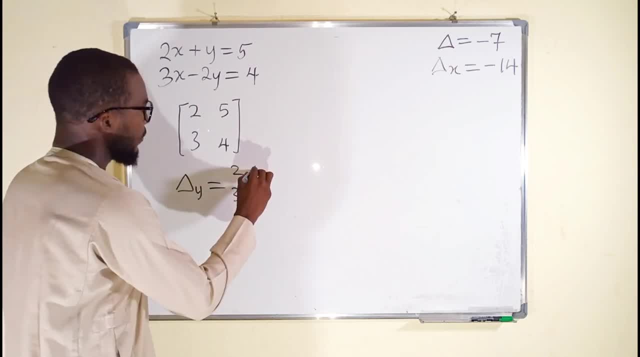 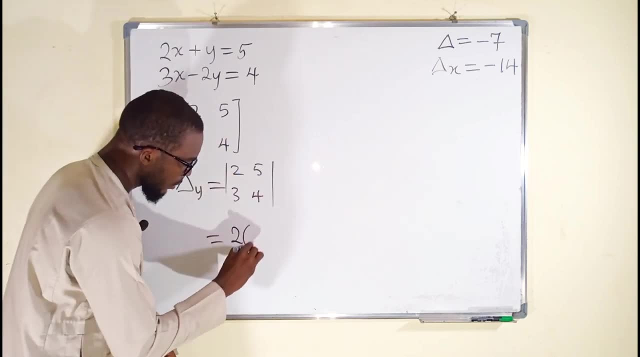 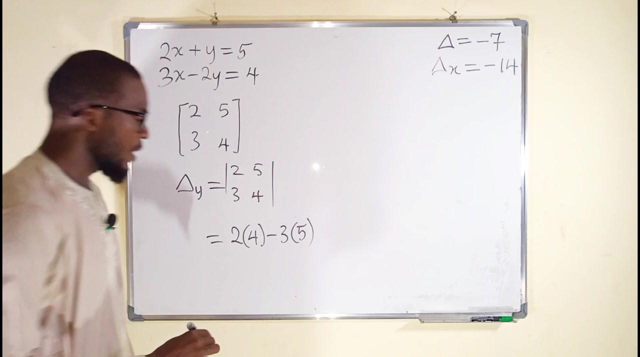 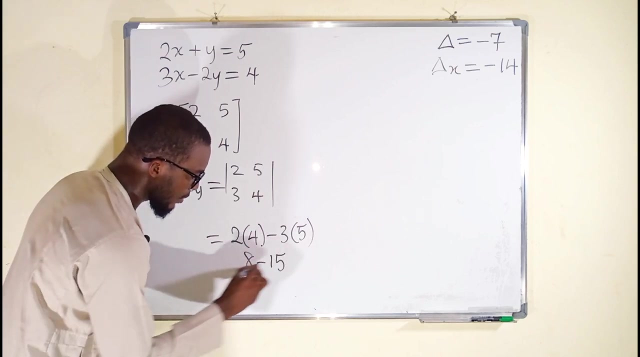 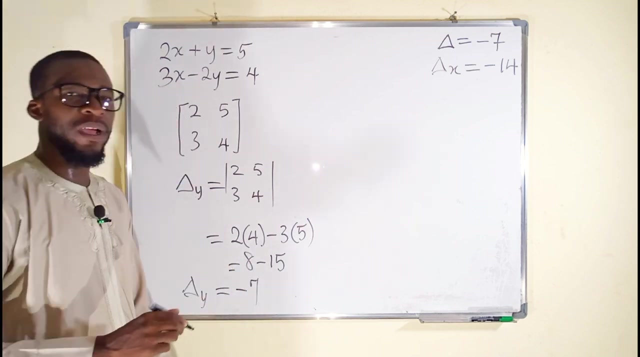 will be two, three, five, four. two multiplied by four minus three multiplied by five. let's simplify: we have 2 times 4, 8, minus 3 times 5 is 15.. Finally, determinant with respect to y is equal to negative 7, because 8 minus 15 is negative 7.. 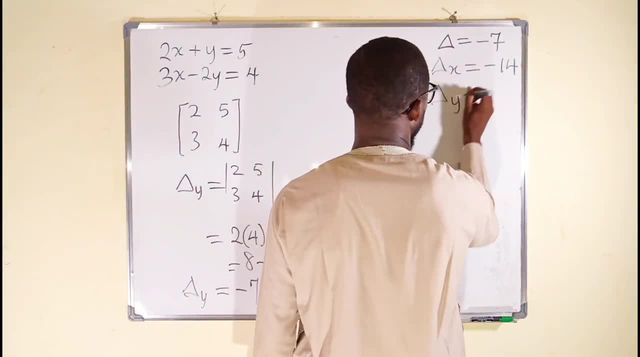 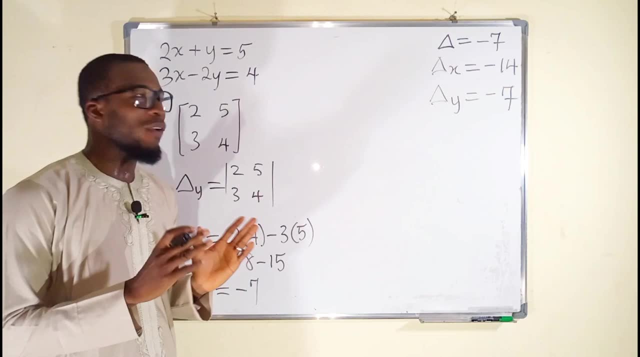 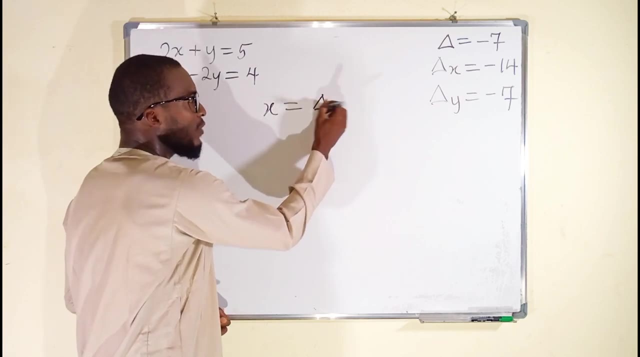 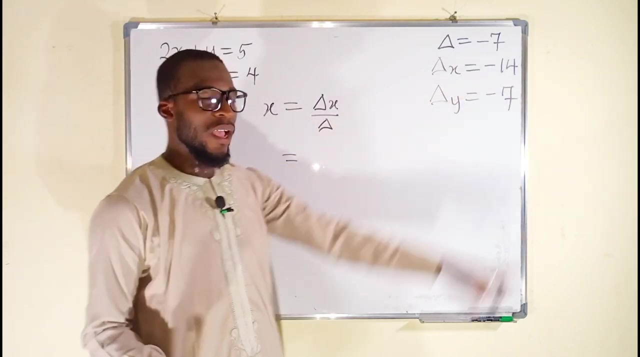 Let us keep it here. So next we want to find the value of x. To find the value of x, we are going to divide the determinant with respect to x over the main determinant. This is equal to. the determinant with respect to x is negative 14.. 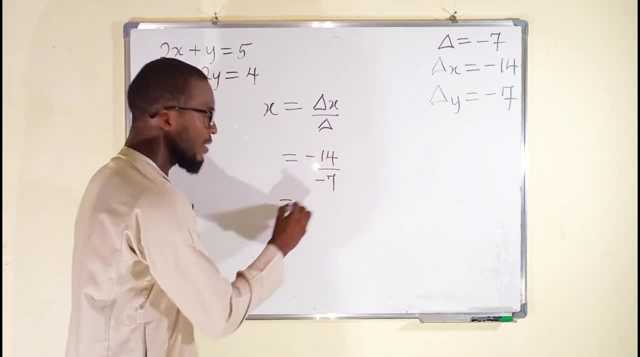 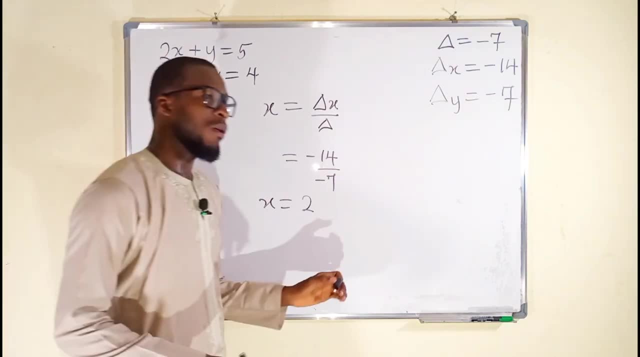 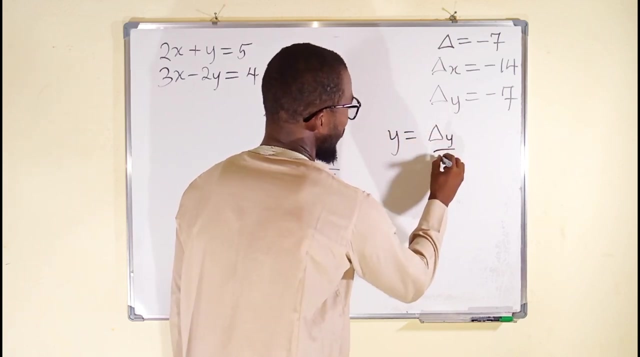 The main determinant is negative, 7. And negative negative cancels 14 divided by 7 is 2. And hence x is equal to 2.. To find the value of y, we say that the determinant with respect to y divided by the main determinant 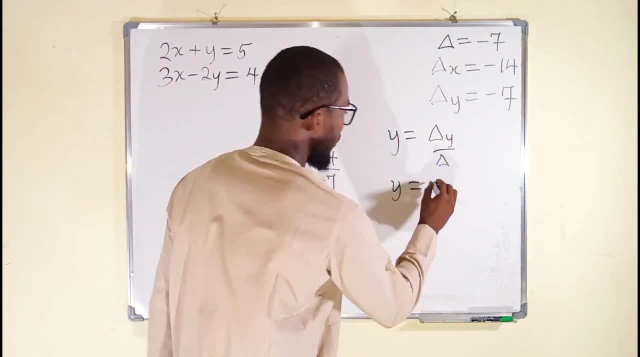 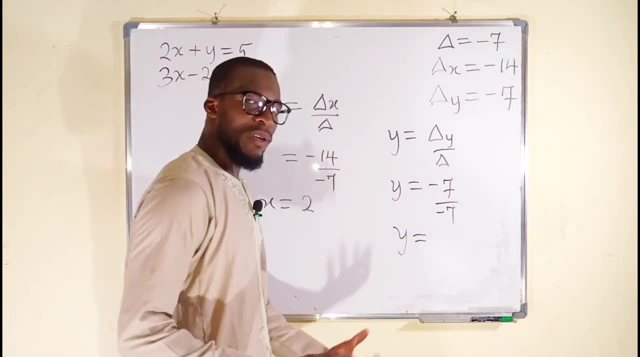 y is equal to the determinant with respect to y is negative. 7. Main determinant is also negative 7. Negative 7 divided by negative 7 is equal to 1.. So x is equal to 2 and y is equal to 1.. 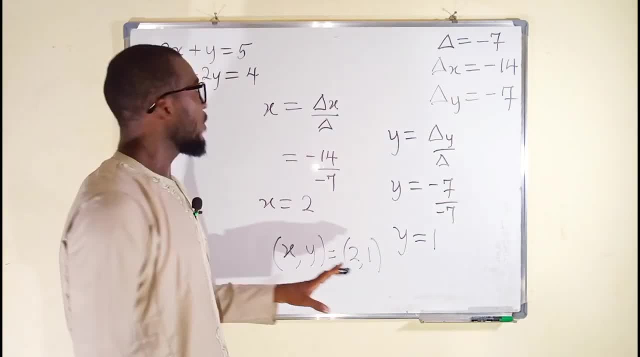 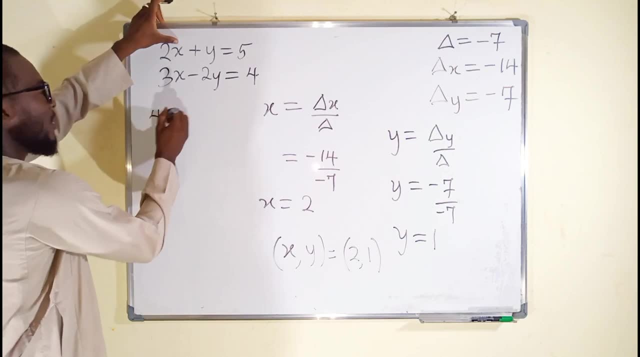 You can check this in the main equation. The main equation is 2 multiplied by x. the first equation, Meaning 2 multiplied by 2, you can see- is 4.. Then you add: y is equal to 1.. Is this equal to 5?? 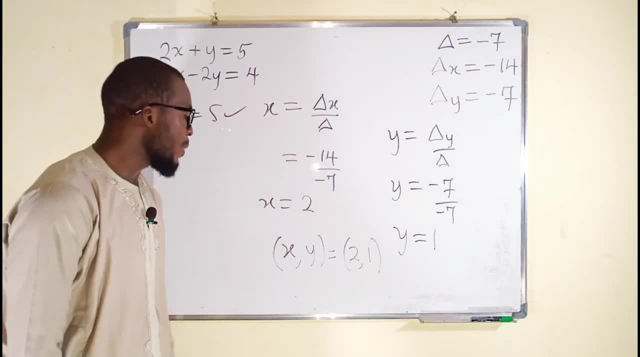 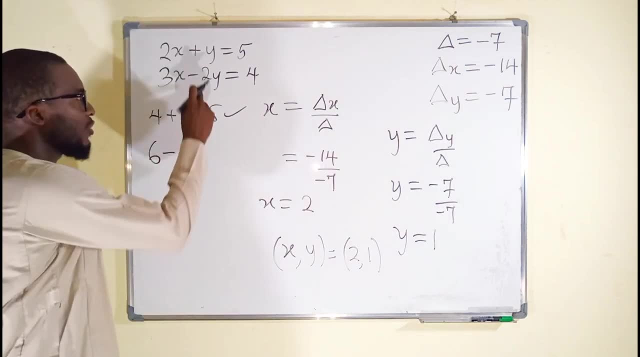 Yes, absolutely, because the right hand side is equal to 5.. To test the other equation, we have 3 multiplied by x, 3 multiplied by 2, which is 6.. Then you subtract 2 multiplied by y, 2 multiplied by 1, which is the same thing as 2.. 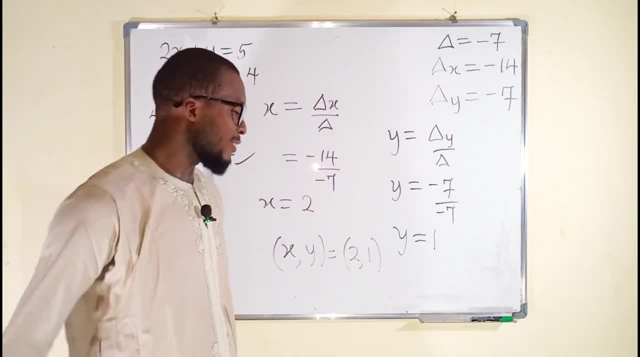 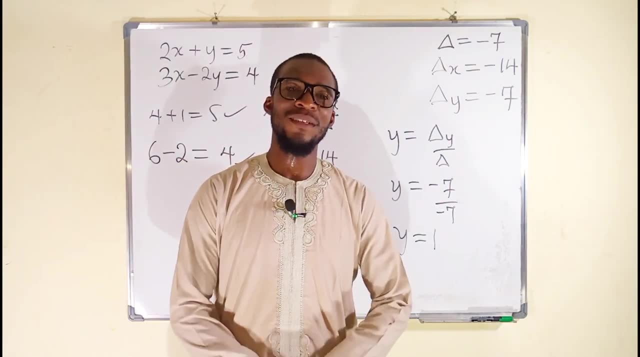 Is this equal to 4?? Absolutely, And hence x is equal to 2 and y is equal to 1.. This is all I have for you today. Thank you for watching and you have a nice day.